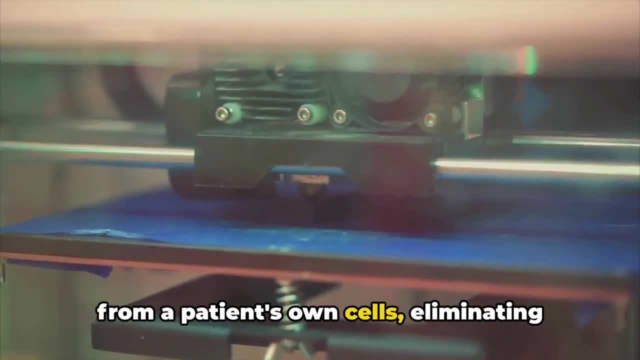 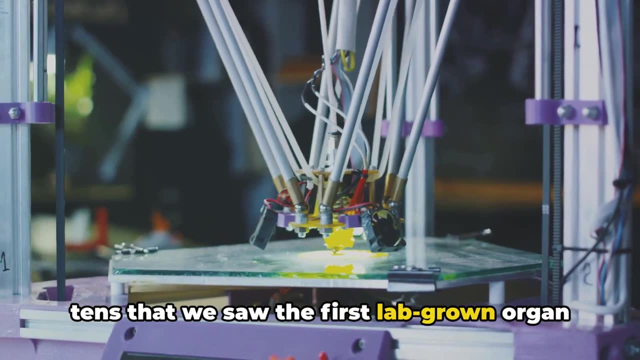 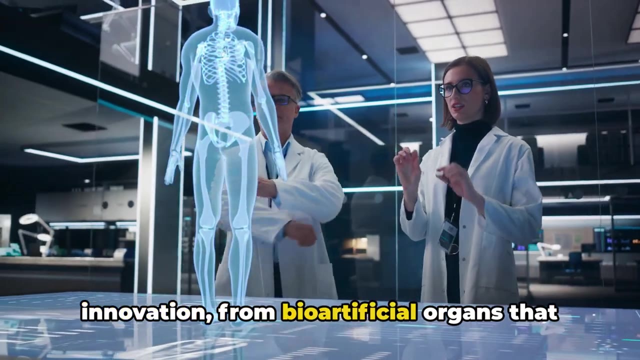 where organs could be printed layer by layer from a patient's own cells, eliminating the risk of rejection. However, it wasn't until the 2010s that we saw the first lab-grown organ transplants, a major milestone in the field. The last decade has seen a flurry of innovation from bioartificial 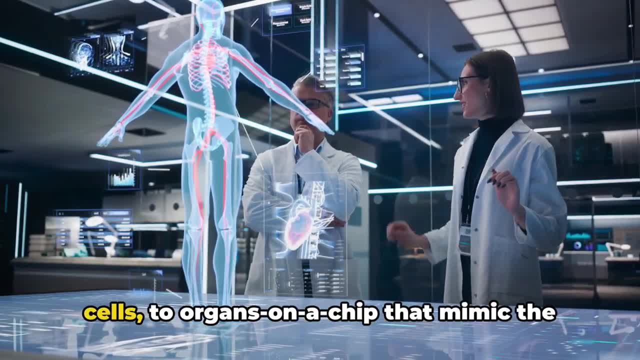 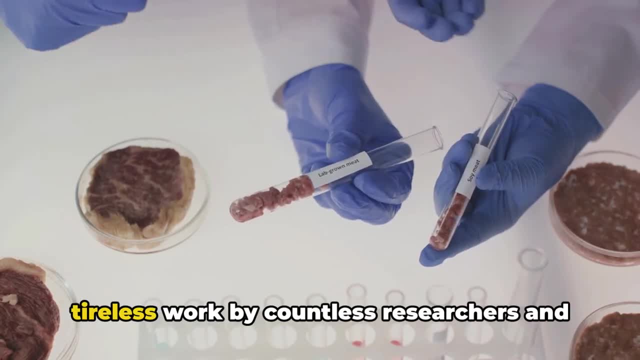 organs that combine synthetic materials with living cells to organs on a chip that mimic the function of human cells. The technology has been a key part of the development of artificial organs. The technology has been a key part of the development of artificial organs. These advancements are the result of tireless 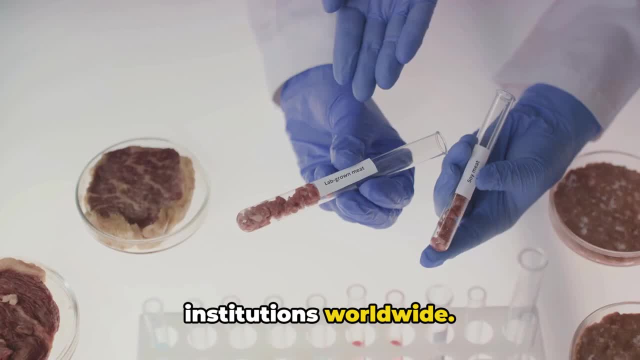 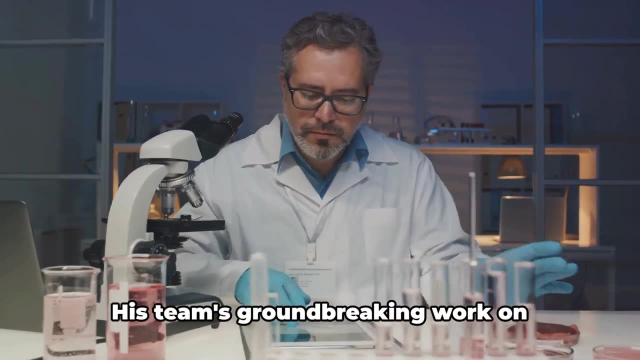 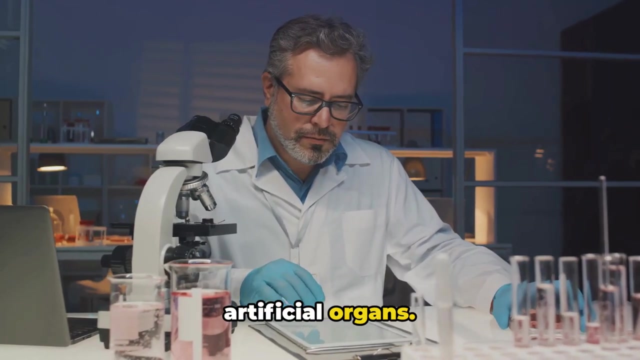 work by countless researchers and institutions worldwide. Among these, Dr Anthony Atala from the Wake Forest Institute for Regenerative Medicine stands out. His team's groundbreaking work on lab-grown bladder transplants has set the stage for the next generation of artificial organs. 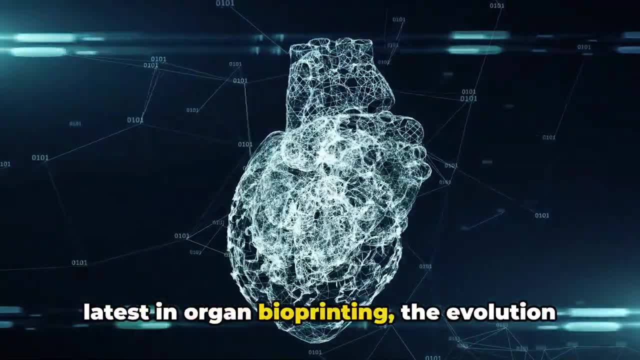 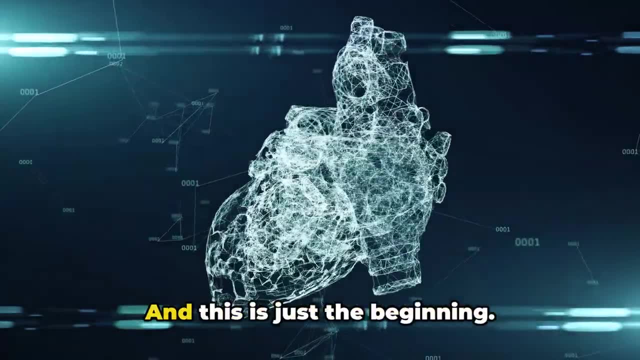 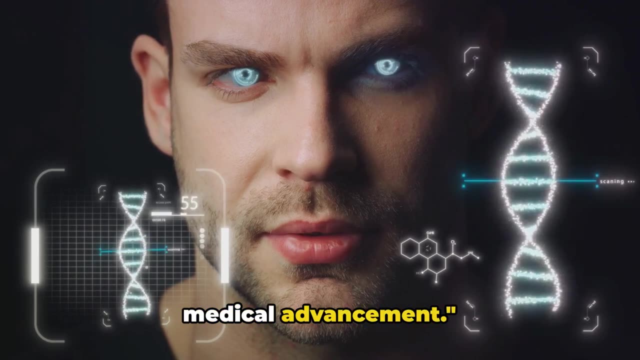 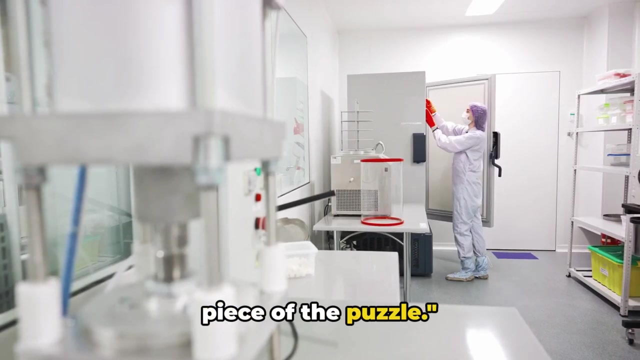 From the first artificial heart to the latest in organ bioprinting, the evolution of artificial organs has been a journey of order. This isn't just about the strength of artificial organs, and if you look at the body, you can also see an abundance of tissue and tissue engineering. Tissue engineering is 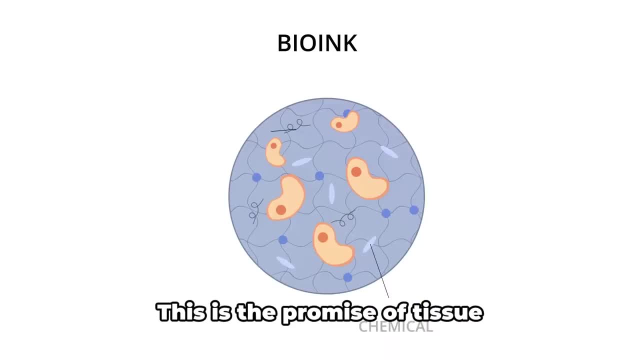 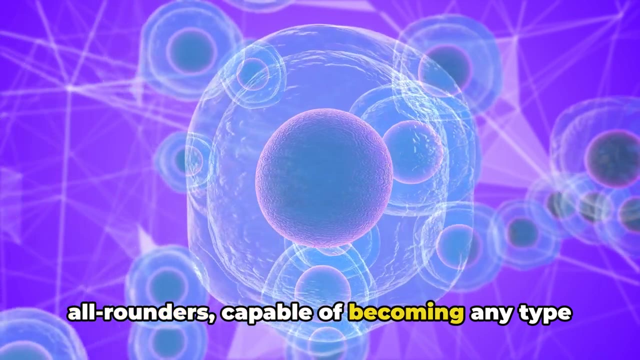 another critical piece of the puzzle. Imagine a world where we can create not just artificial organs, but functional tissues right in a lab. This is the promise of tissue: create living, functional tissues. the process begins with cells. these are often stem cells, the body's all-rounders, capable of becoming any type of cell. these cells are then placed onto a 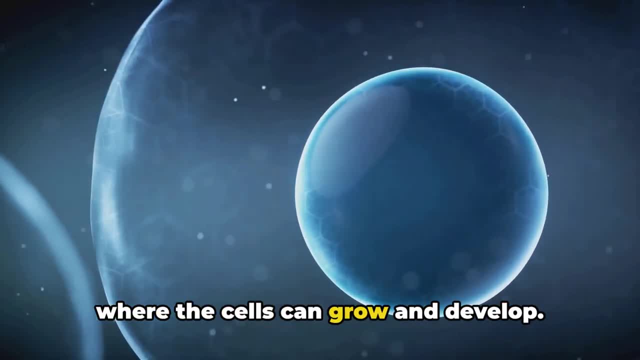 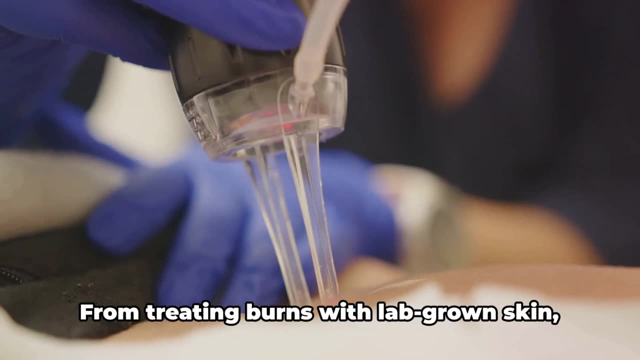 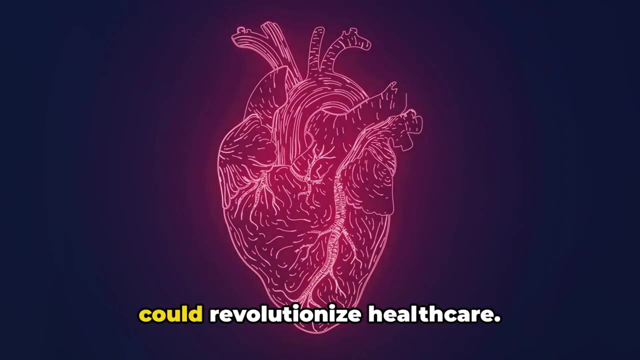 scaffold, a structure that provides a home where the cells can grow and develop. the result: tissues that can mimic those found in the body. the potential applications are vast, from treating burns with lab-grown skin to replacing damaged heart tissues with new, healthy ones. tissue engineering could revolutionize healthcare. it even offers hope for diseases currently considered. 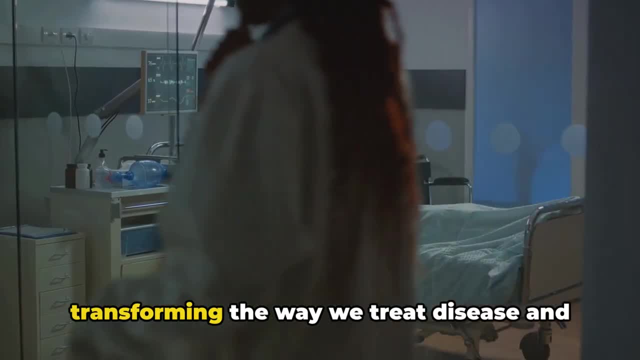 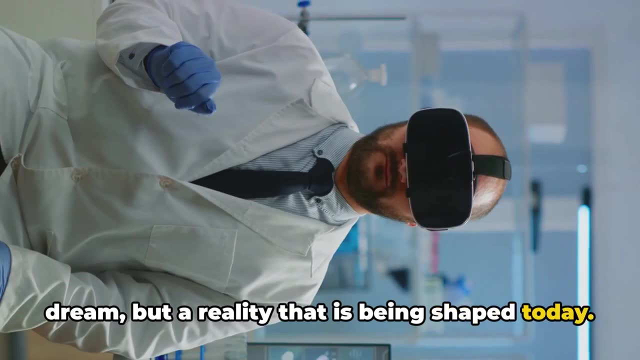 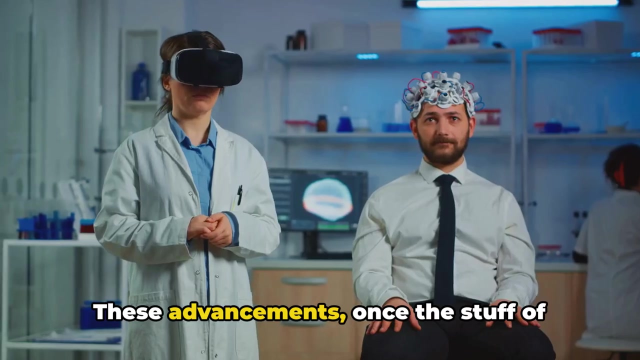 incurable. tissue engineering holds the promise of transforming the way we treat disease and repair the human body. the future of medicine is not a distant dream, but a reality that is being shaped today. the potential of artificial organs and tissue engineering to revolutionize healthcare is immense. these advancements, once the stuff of science fiction, now stand poised to redefine the